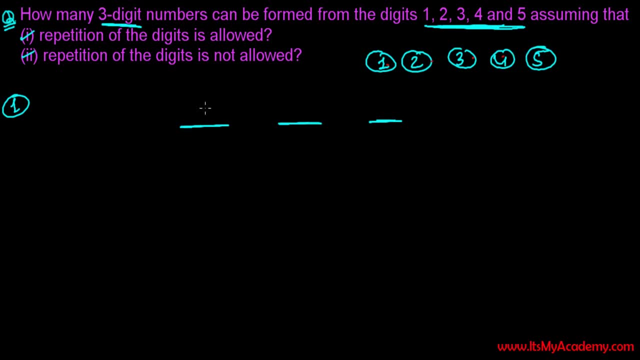 write any one out of these five digits, All right. so there are five possible ways to select, All right. and since repetition is allowed, if I'm writing here one, next time also I can write here one, because repetition is allowed. So let's do the first one. So let's do the first one. So let's. 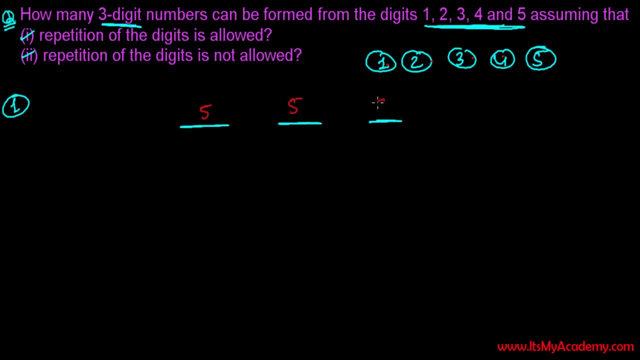 say, this is allowed in the first case, So this can be also written five times, and this can be also written five times. So five times five times five, It means 125 numbers. are there All right? so how many three digit numbers can be formed? They can be formed 125 numbers if the repetition of the 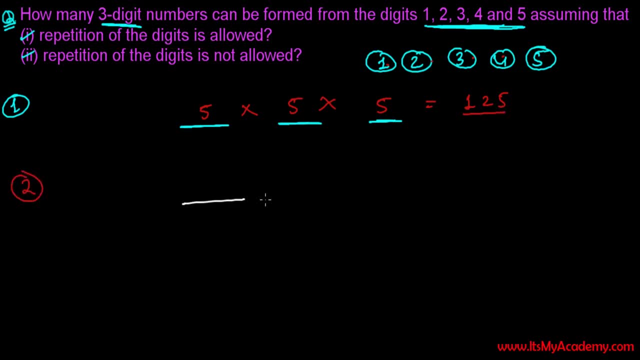 digits is allowed. Let's go for the second question. So in the second case also, we have to write three digit number and the repetition is allowed this time. keep in mind. So the first. the selection of the first number is very easy because we can choose any one. I can say I can choose one, that's. 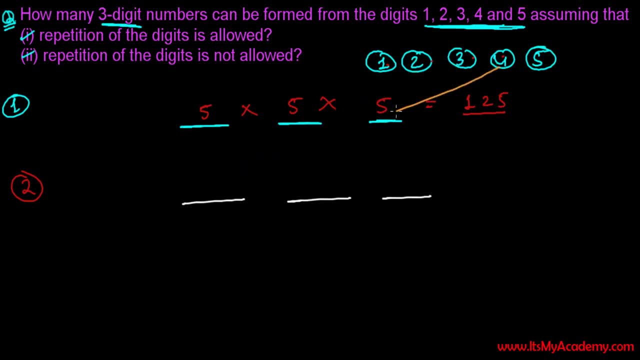 choose one, i can choose two, i can choose three, i can choose four, i can choose five for the first position. so there are five ways to write the first one, all right. so i can choose anyone. let's say, for a while i write here one, just for supposition. all right, so one is dead now. so we have only four. 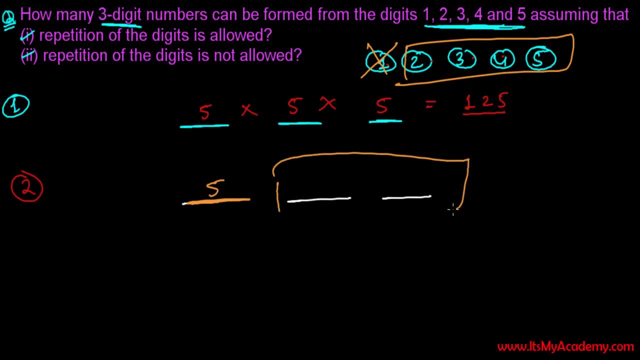 number, because i have written one and i have two space to be filled with rest of the four digits. so this can be written in four ways: it can be two, it can be three, it can be four, it can be five, anyone, it can be all right. and now the third one, third one. before writing third one, let's say we 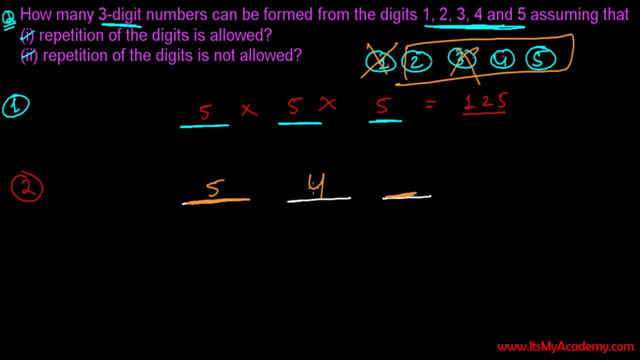 have right. we have written yes, one, any one of them. let's say for a while, three right here. so we have now three options: one, two, three. so with these three options we have to fill the last one position. so there are three options to fill this position. it may be two, it may be four, it may be five all. 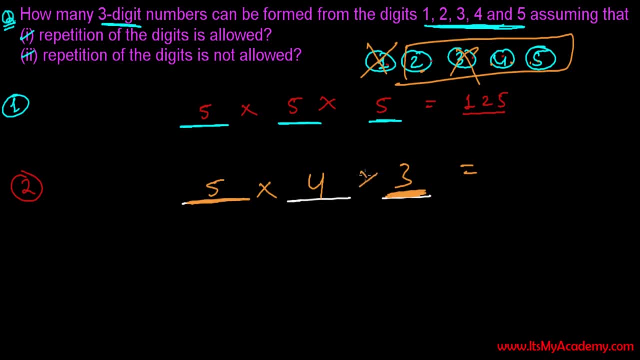 right. so if repetition is not allowed, then five times four times three, five, fours are twenty, twenty times three, sixty. all right, so there are sixty numbers that can be formed, five from these. one, two, three, four, five, if repetition of the digits is not allowed. i hope you understand. 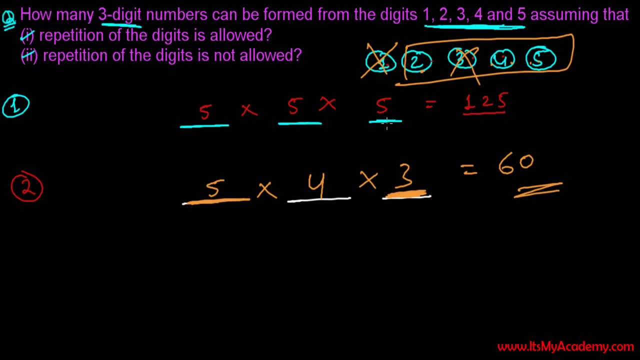 it. if there is any more confusion, any doubt, then please feel free to comment below this video. i'll definitely get back to you and please, till the time, please like this video and subscribe the channel. i'll be really, really happy to see you guys into the next video with next concept. bye.